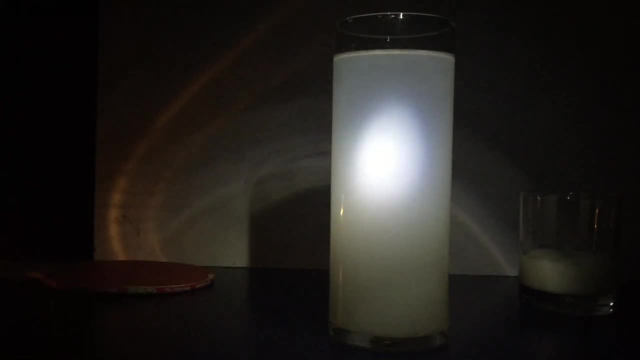 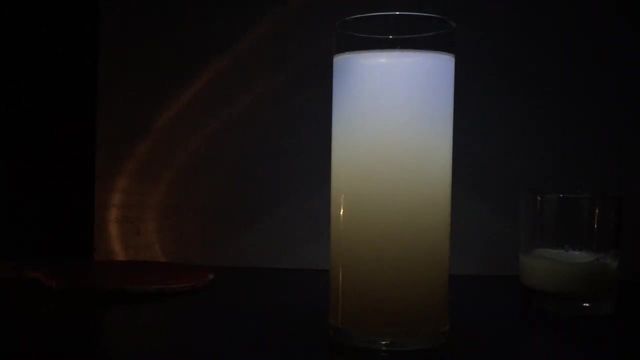 like dust or ash. the light is scattered by the edges of the particles. Now I've switched from a tub to a flower vase or a large glass and you can see with the same liquid, with the milk and water, that the white light on top is showing you more of a blue color. 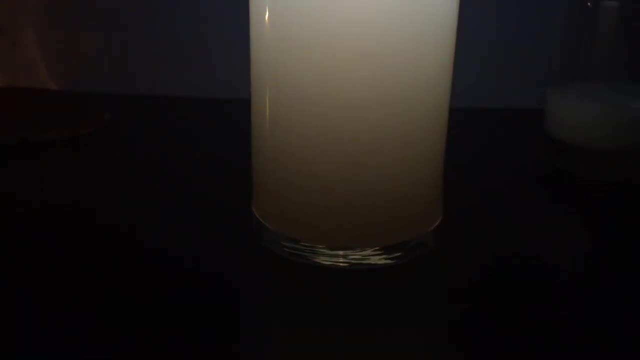 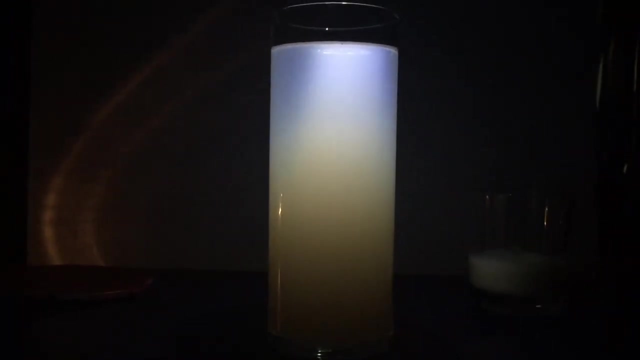 but as it farther, goes down and hits particles, it's more of an orange color. Milk is a colloid which contains tiny particles of fat and protein. When I mix it in the water, I can see the particles scattered in the light as much as the dust scatters light in the atmosphere. 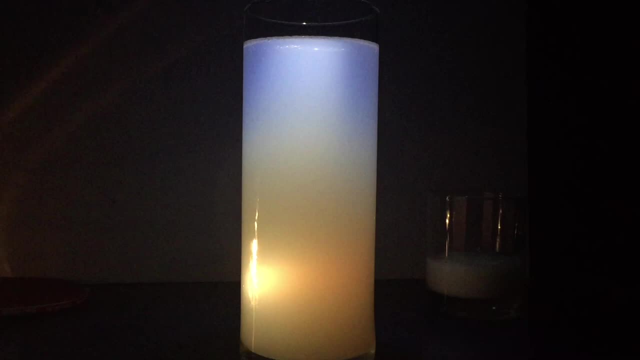 Light is scattered differently depending on its color and light wave. Blue light is scattered the most, while orange and red light is scattered the least. Looking at the daytime sky is like viewing a flashlight beam. from the side, You see scattered blue light. Looking at the sunrise or the sunset is like directly into the beam of the. 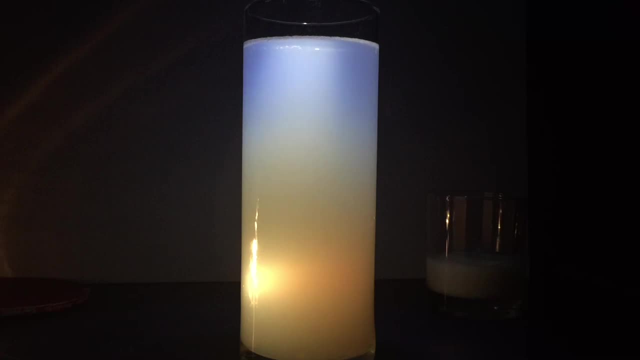 flashlight, but the light hasn't scattered, which is orange and red. Well, what makes the sunrise and sunset different from the daytime sky? Well, it's the amount of atmosphere in the sunlight that has to cross before and reaches our eyes. If you think of the atmosphere, 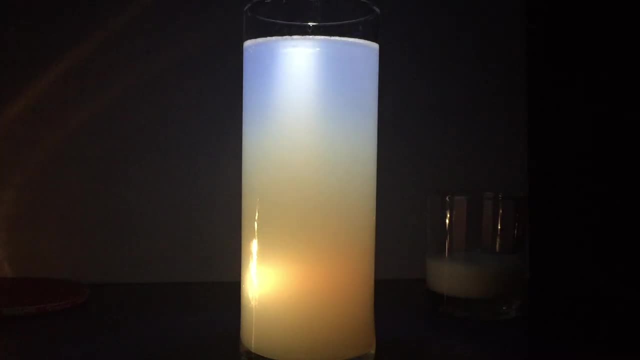 as a coating covering the earth. the sunlight at noon passes the thinnest part of the coating. The sunlight in the sunrise and the sunset has to take a sideways path to that same point through a lot more coating, which means there's a lot more particles that can scatter the 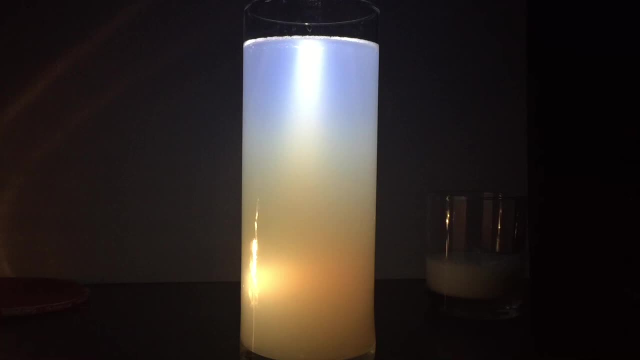 light. If you give this a try at home. I started off with a fourth of a cup of milk, but maybe start off with an eighth of a cup of milk. See what kind of colors you get with the blues and the oranges, and then add a little bit. 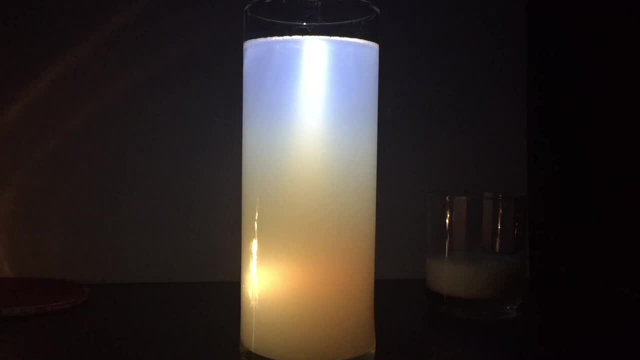 more milk and even go up above a quarter cup to see if you actually increase the orange or the reds or increase the blues. So when you do that, make sure you comment back and let me know what you saw. I appreciate that. I hope you enjoyed this video. Remember to 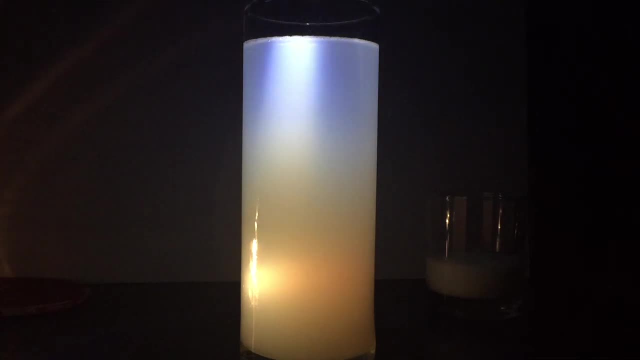 click thumbs up and to subscribe, and thanks for watching. Subtitles by the Amaraorg community.